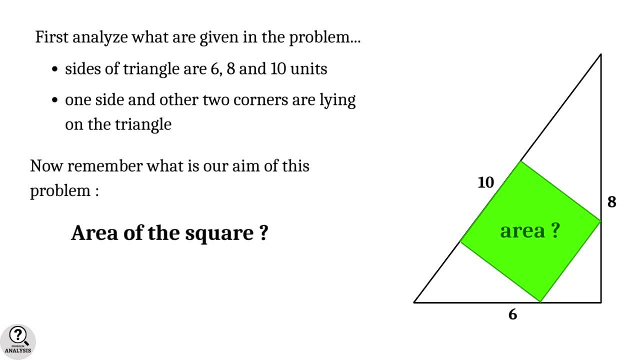 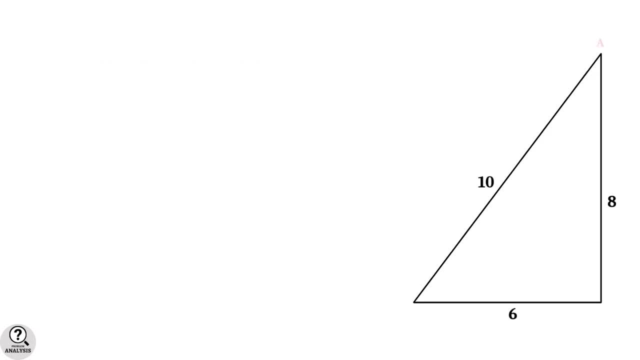 here, It is nothing but to find the area of the square. This is the structure of our problem, So always keep in mind. For better understanding, let's denote the triangle by ABC. Now I have a question: Can you find anything special about this triangle? We know that. 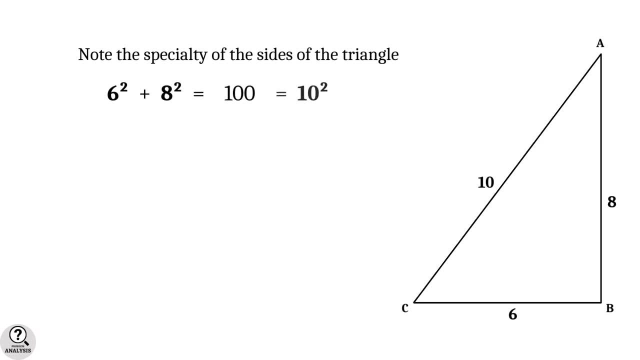 6 square plus 8 square, equal to 100, which is equal to 10 square. What does it mean? The sides of the triangle obey Pythagoras' theorem, Which means the sides of the triangle are the same as the sides of the triangle. The sides of the triangle are the same as. 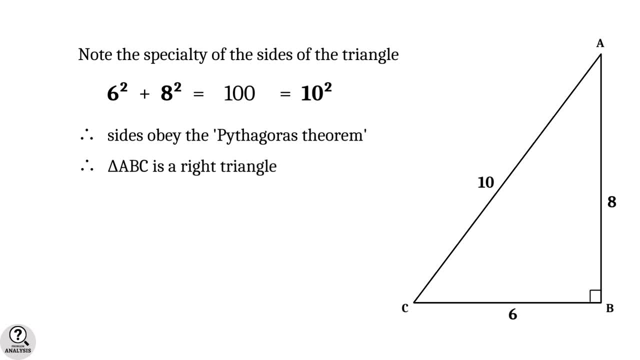 the sides of the triangle. The sides of the triangle are the same as the sides of the triangle. The triangle ABC is a right triangle. Note that we have three more right triangles in the actual figure. Now let's take angle A, equal to x degree. Therefore, angle C will 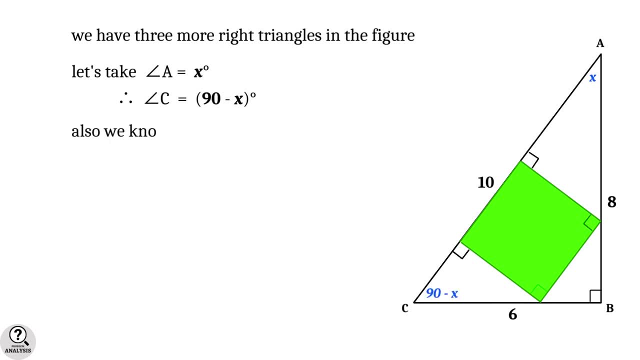 be 90 minus x degree. Also, we know that the angles inside the square are 90 degree each. Using this, calculate the remaining angles also. Then we get like this: Now compare all the right triangles we have. As you can see, all of them have equal angles. So we have. 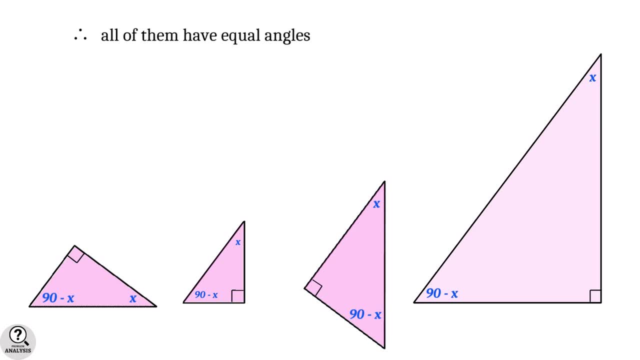 x degree, 90 degree and 90 minus x degree. What does it mean? If two triangles have equal set of angles, then they are similar triangles. That is here. all these four triangles are similar triangles And therefore, by the property of similar triangles, the ratio of 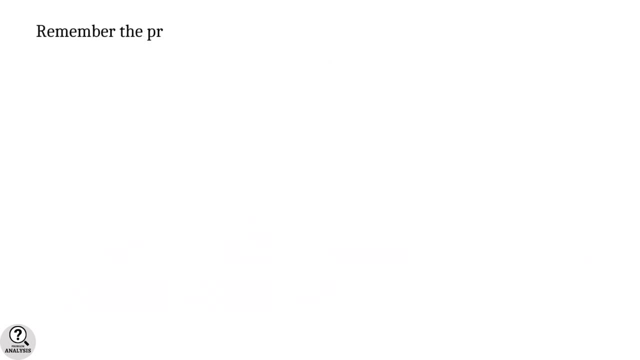 similar sides are equal. Before proceeding, remember the important properties of similar triangles. If we have two triangles which are similar, then they are equal. So we have two triangles which are similar to each other, Then the first property is that both the 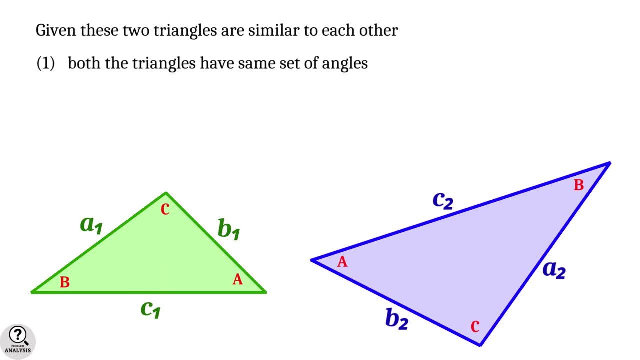 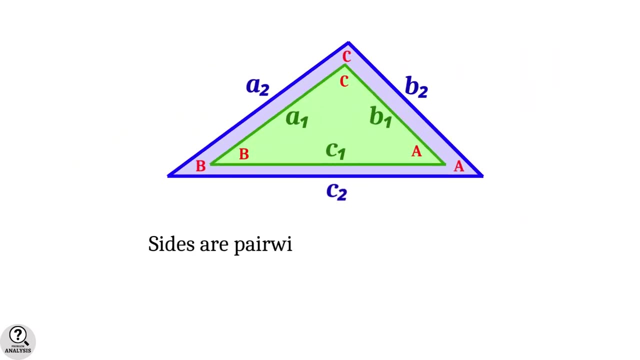 triangles have the same set of angles, And the second property is that the ratios of similar sides will be equal. That is, the ratios a1 by a2, b1 by b2 and c1 by c2 are equal. Geometrically, we can place these triangles, as the sides become pairwise, parallel to each. 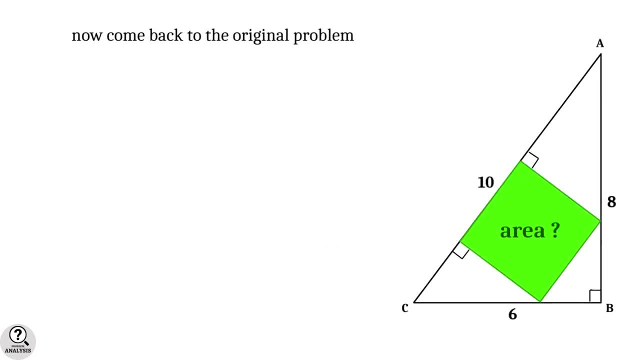 other. Now come back to the original problem. Let's denote the square as PQRS And PQRS can take the side length of the square as a units. Now consider the similar triangles: Triangle ABC and triangle AQR. Taking the ratios of similar sides, we get QR by QA equal.